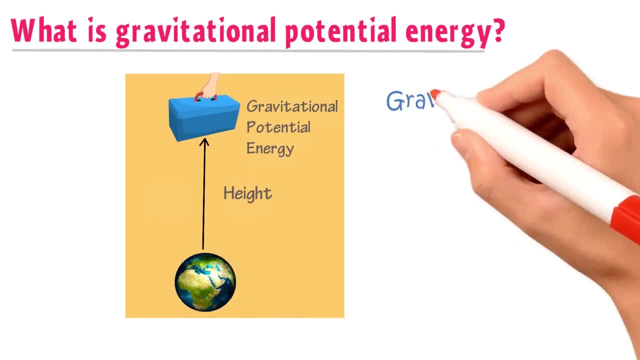 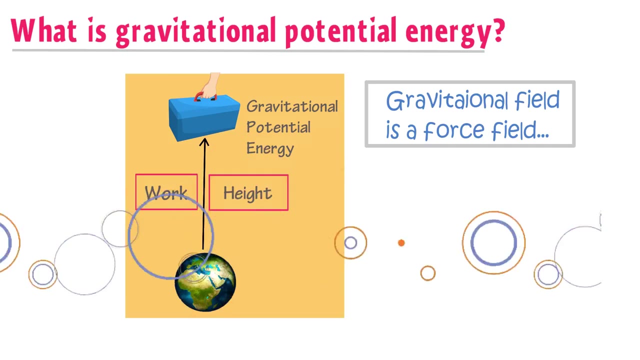 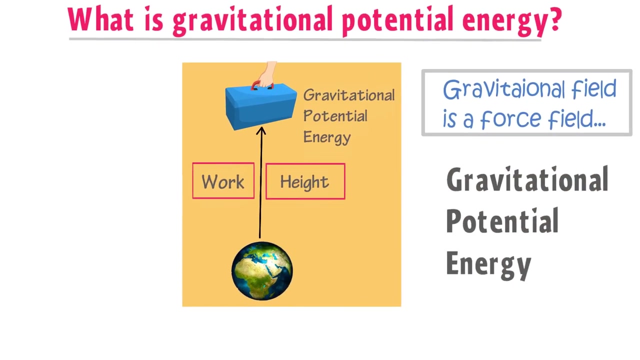 body above the earth's surface. As we know that gravitational field is a force field, when you do some sort of work on a body and change the height of the body, then this work against gravity stores in the body as a gravitational potential energy. That's why I told you that potential energy is also known as a stored form of energy. 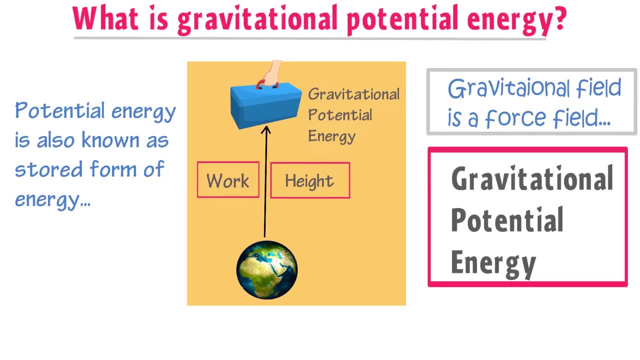 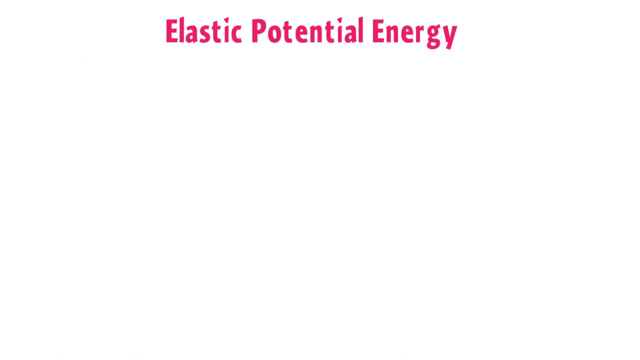 Thus remember that gravitational potential energy only exists when an object is at a particular height above the earth's surface. The another example of potential energy is elastic potential energy. If an object possesses a particular height above the earth's surface, it will be due to the change in position or configuration. 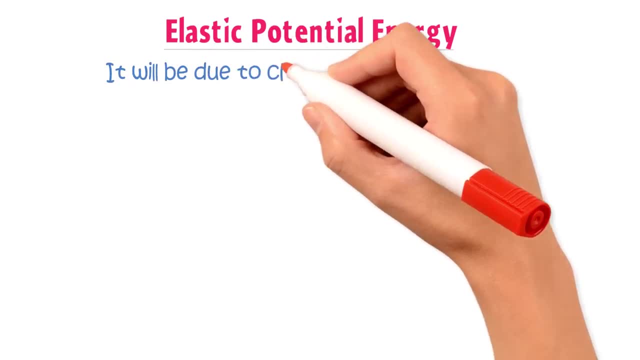 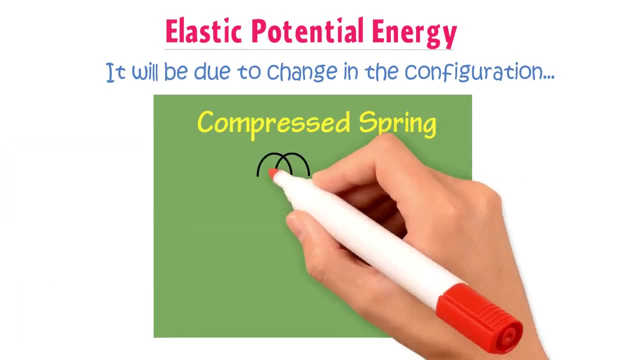 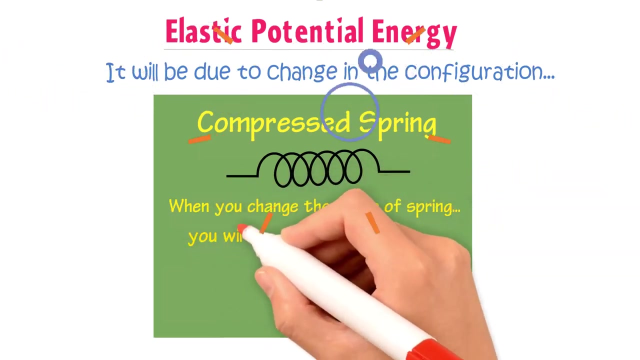 The other example of potential energy is elastic potential energy. This is elastic potential energy. It will be due to change in the configuration. The best example of elastic potential energy is compressed spring. When you change the shape of a spring, you will need to do some sort of work. 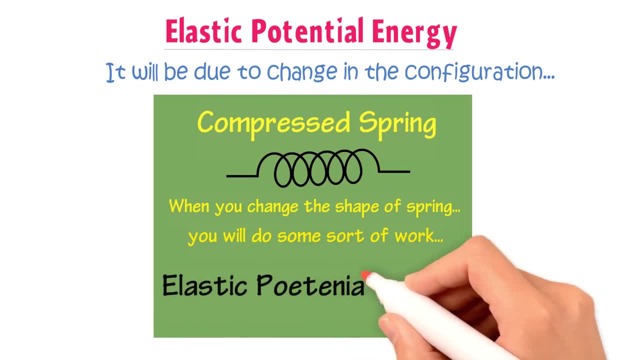 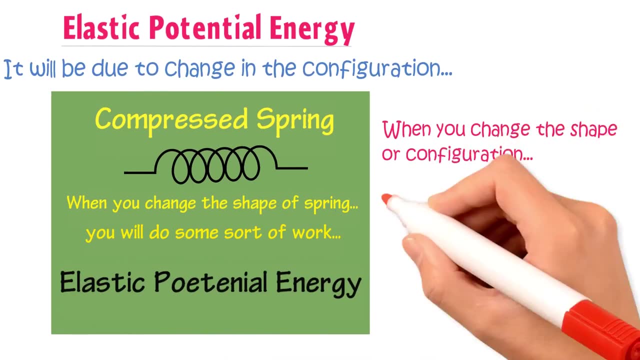 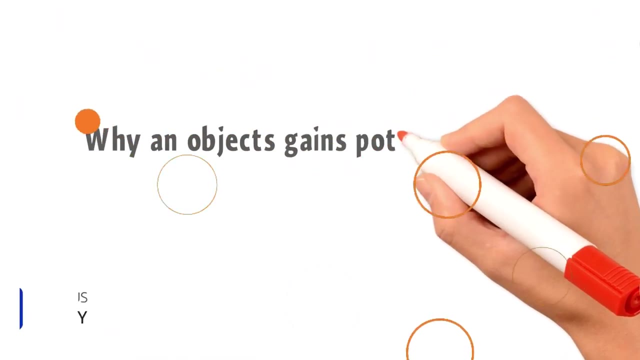 This work will be stored as elastic potential energy in the spring. Thus, remember that when you change the shape or configuration of the spring you will need of a body, the body will gain elastic potential energy. why an object gains potential energy when you change its position, our configuration. well, it is. 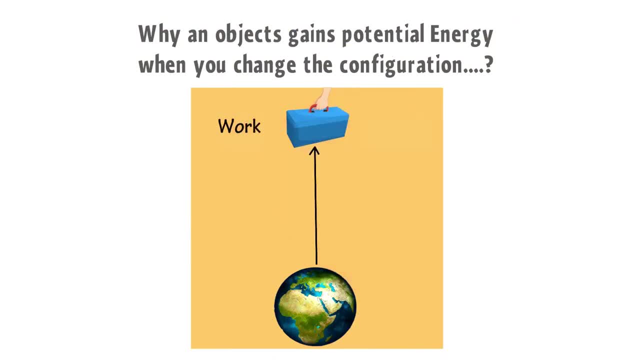 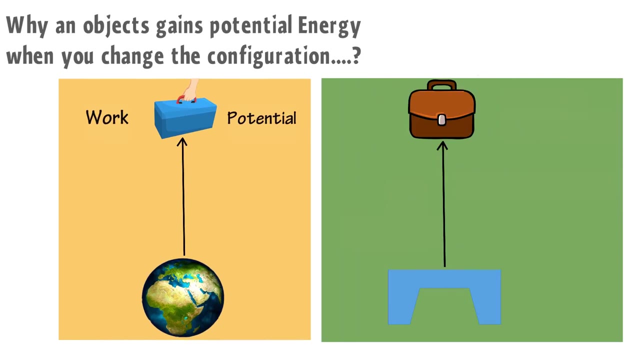 due to the work we do on objects. as a result, this work stores within the objects and they have then potential to do work. for example, when you left an object above the table, you exert force and the object also cover a displacement in the direction of your force. according to physics, were done is equal to F dot. 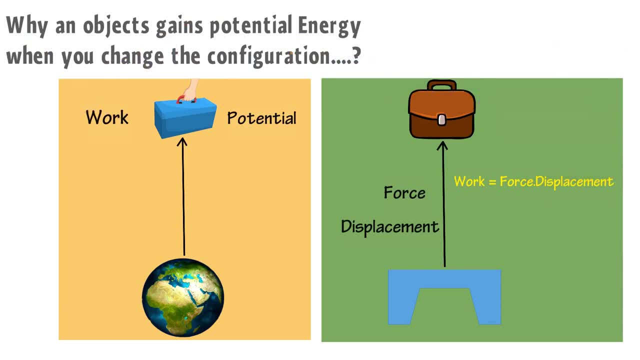 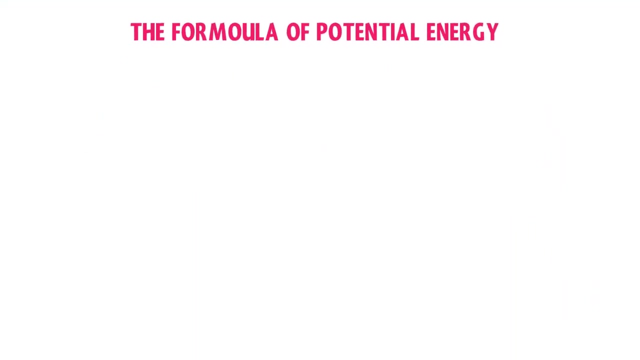 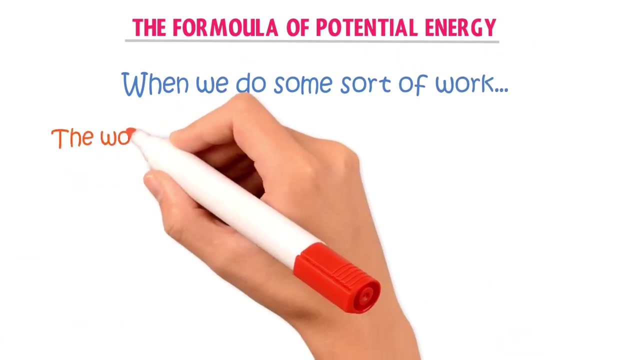 displacement. it means you have done some sort of work while lifting this object above the table. hence, this work stores potential energy in the object. we call this energy as a gravitational potential energy. now let me derive the formula of a potential energy. as we learned, when we do some sort of work on an object and this word and change the position or 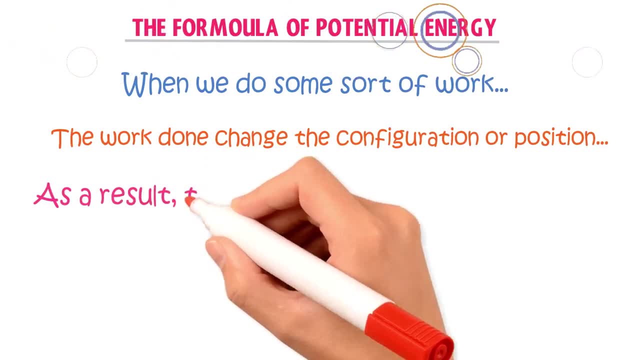 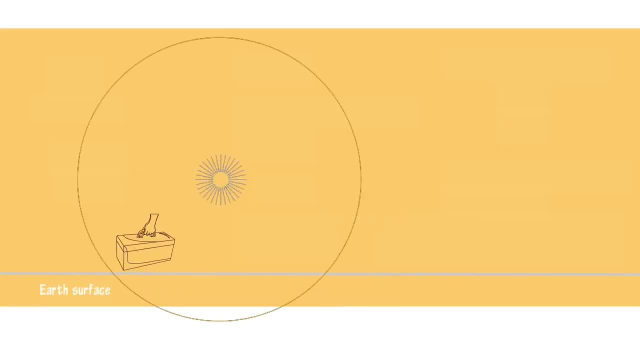 connection between the object and the object we call gravitational potential energy. we say that the body then possesses potential energy. for example, when you left in an object above the earth's surface, you do some sort of work in, the object gains a particular height, H, due to the force F you exert. hence were done. 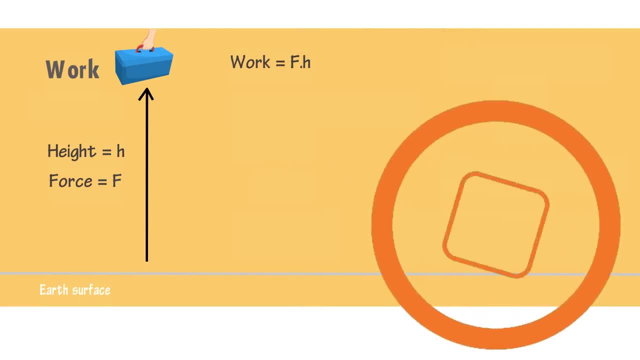 is equal to force dot displacement. as we learned in the previous lesson, we can show the Or we can say that Vrdan is also equal to energy. Here the energy gained by a body is potential energy or Vrdan is equal to potential energy. 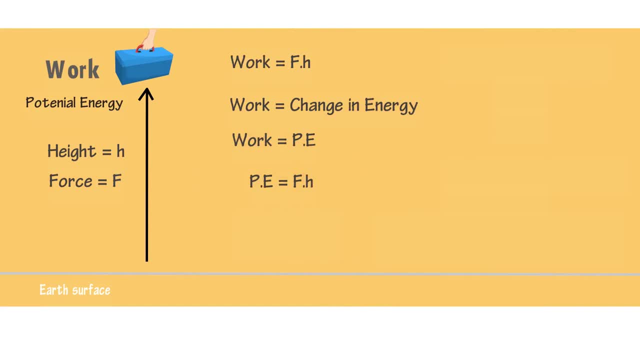 Hence potential energy is equal to force. dot displacement. According to Newton's second law, F is equal to ma, where acceleration a is replaced by g. By g, V means gravitational acceleration. Hence F is equal to mg. Now putting the values and we get potential energy is equal to mgh. 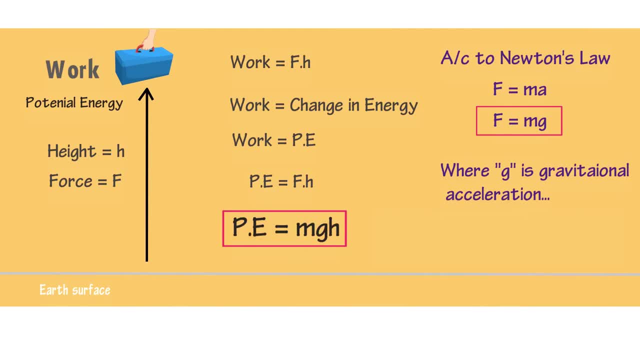 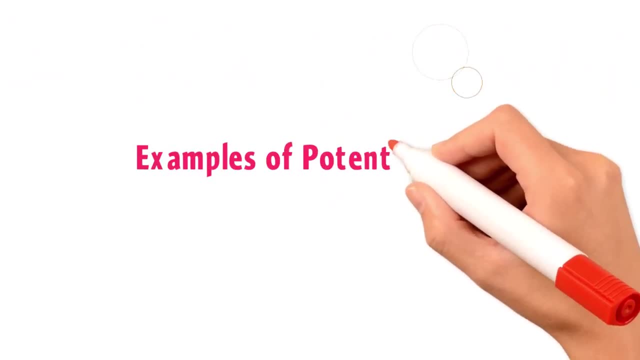 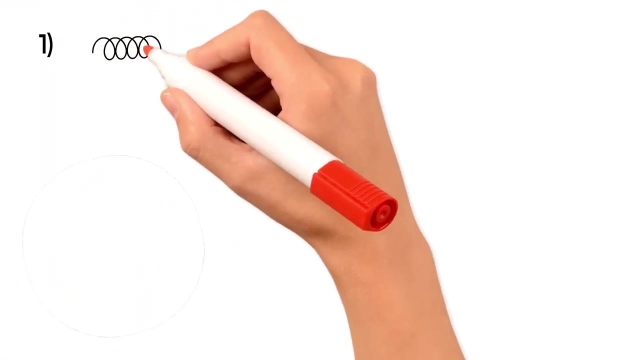 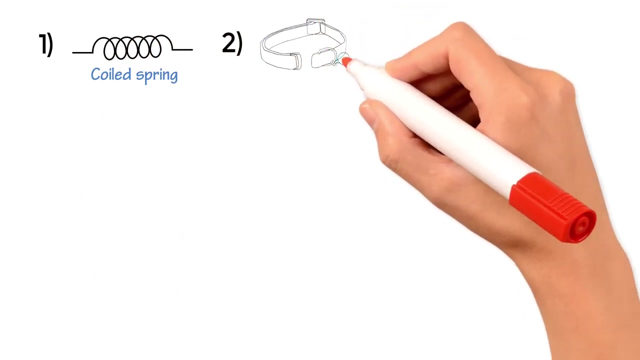 This is the formula of potential energy. The SI unit of potential energy is Joule. At last, let me give you some other examples of potential energy. Number one: a coiled spring has potential energy. Number two: a stretched rubber band has potential energy.